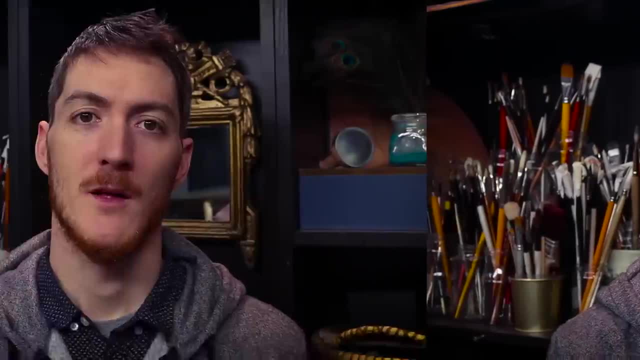 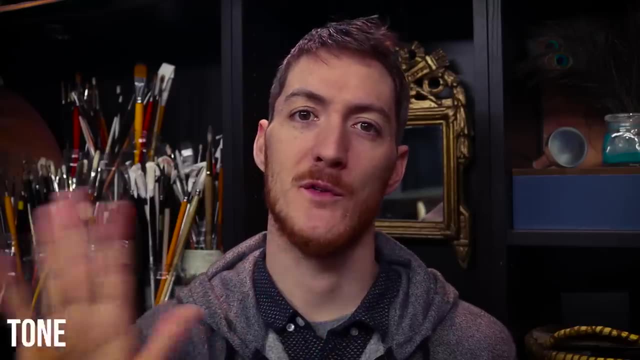 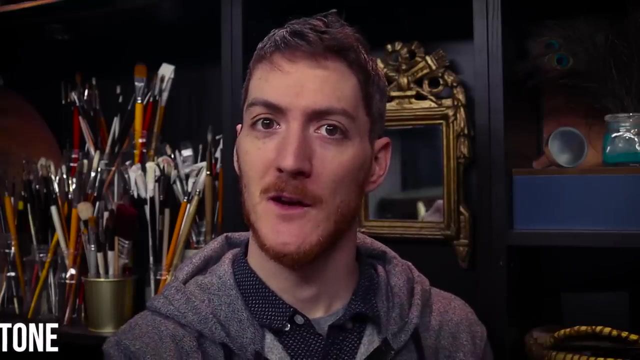 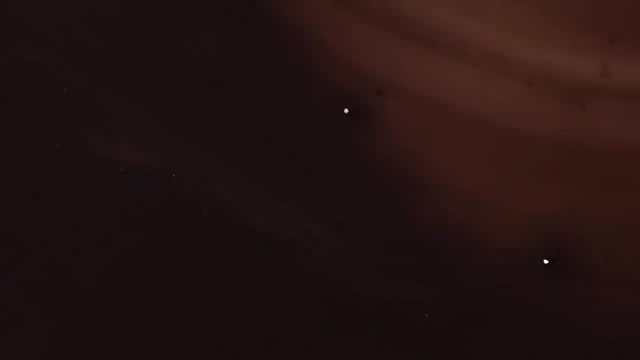 a good idea of where everything should be the placement. The next objective tone is to have some sort of nice unifying tone over the canvas to get rid of the white. Some people like to keep the white canvas during the entire painting, but many artists like to have a nice neutral tone. that sort of makes it easier. 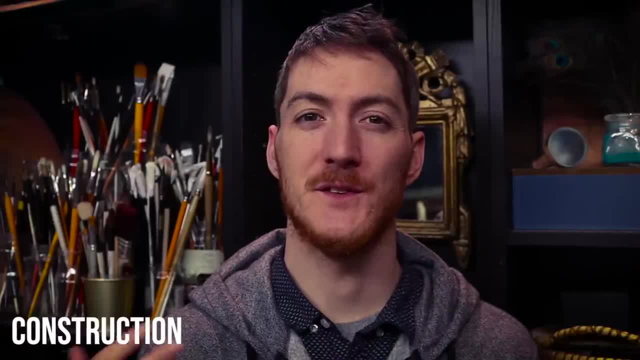 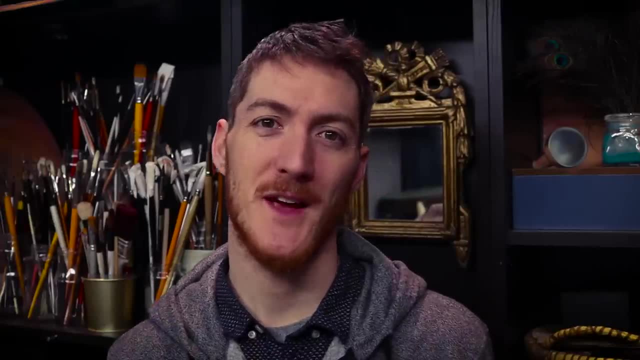 to judge colors. The third is to start the construction of the painting and start elaborating the composition. I'm going to cover 5 different options that you have in the beginning of your painting. Depending on your skill level and what you feel comfortable with, you can start with. 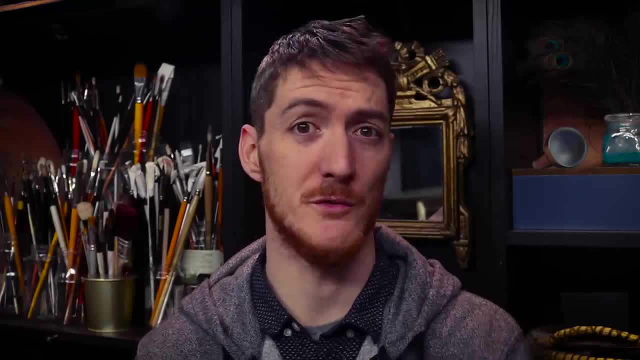 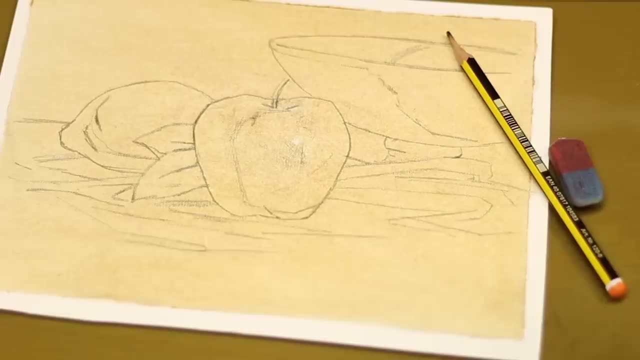 whatever you want to choose. So the first option is to draw with graphite or charcoal. It's the easiest way to draw the outline. The benefit is that it can easily be erased and corrected. One of the big downsides is that dry techniques like graphite or charcoal can be wiped out if you want to create a tone. 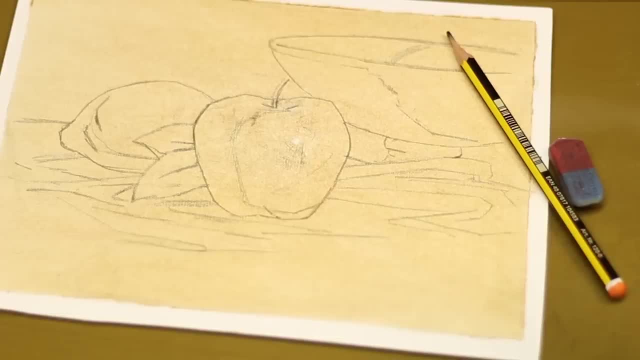 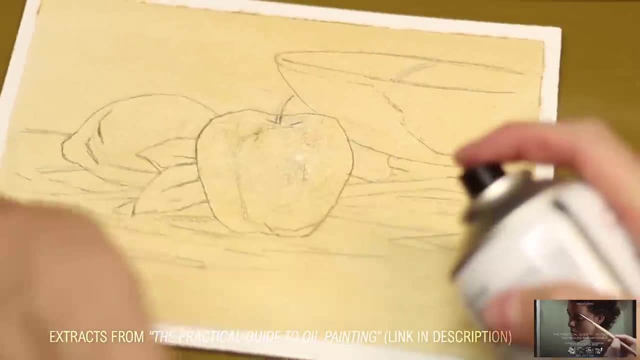 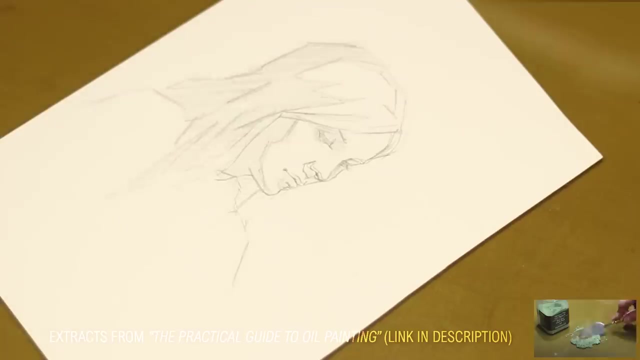 with fluid paint. But don't worry, because you have some options. Option A: you can use fixative. Even if it removes some of it, a subtle outline will still be visible and that's the only thing you need actually. Option B is to not tone. You leave the canvas white and you use a little bit of fixative. 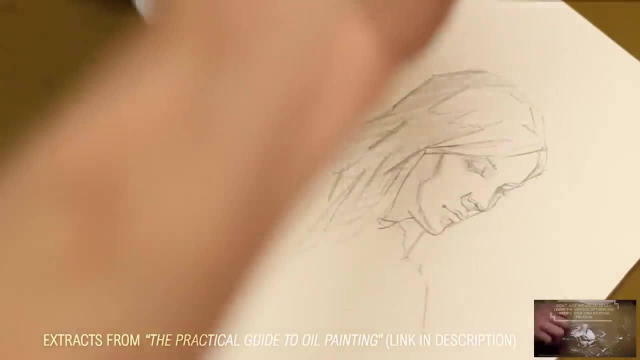 and after that you cover the surface with acrylic matte medium, which is going to seal the surface and prevent the graphite from smudging. So that's the first option. The second option is to use a little bit of fixative and after that you cover the surface with acrylic matte medium, which is going to seal the surface and prevent the graphite from smudging. 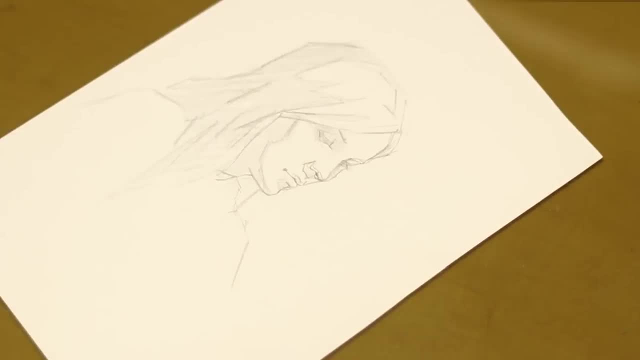 So that's the first option. The second option is to use a little bit of fixative and after that you cover the surface with acrylic matte medium, which is going to seal the surface and prevent the graphite from smudging. And the third option, option C, is to trace over the lines with ink, like Indian ink. 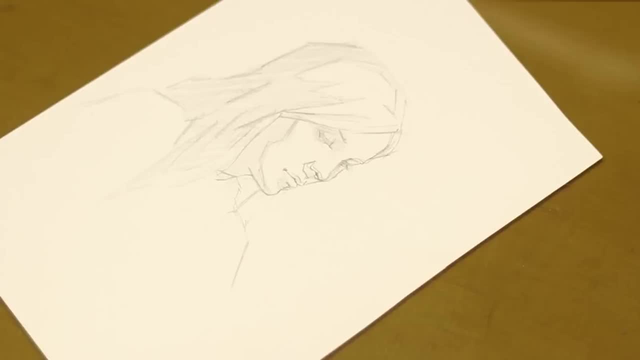 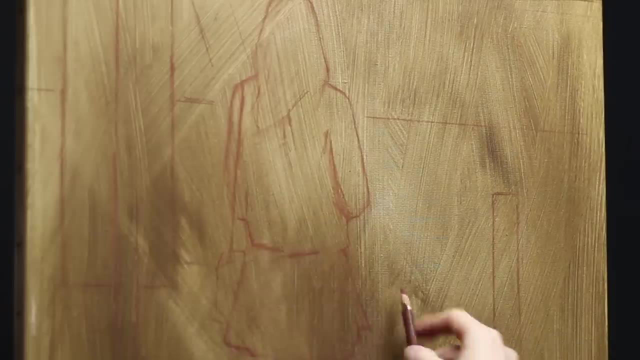 which will not be removed, even if you cover it with fluid paint. Now the second technique is to draw with cutted pencils. Cutted pencils are not like charcoal, because they contain a binder that makes them harder to erase, but the good thing is that they don't smudge or get wiped out by the mineral. 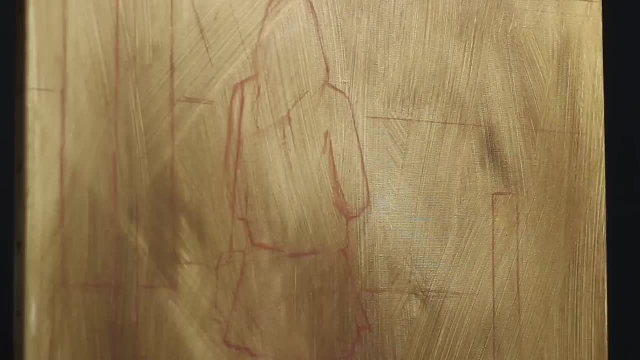 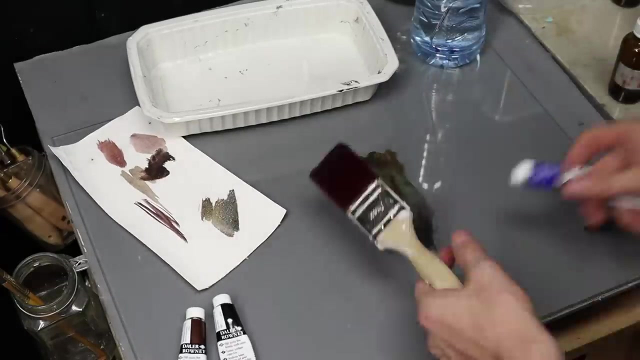 spirits. Plus, you can choose a color that won't be noticed if it smudges. So the downside, though, is that it's hard to remove. The third option is to draw on an acrylic tone. For this option, instead of first doing the outline, you just want to start by covering. 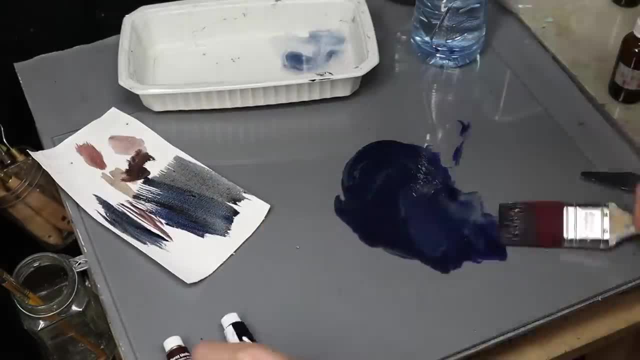 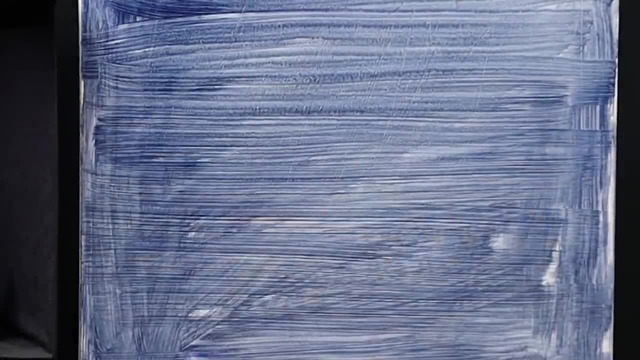 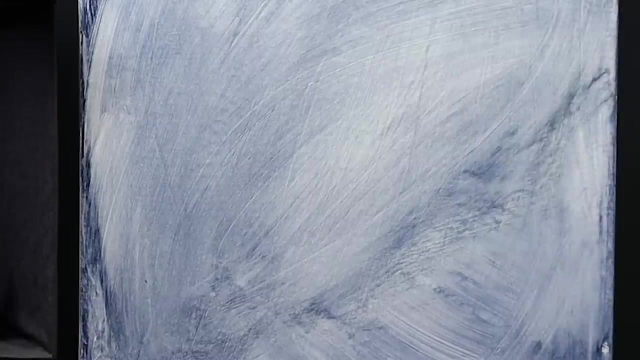 your canvas with whatever color you want for your underpainting, And instead of using oil paint and mineral spirits, you want to use acrylic and water or an acrylic medium. Now, be careful: this method can only be used if you are using universal acrylic gesso. on. 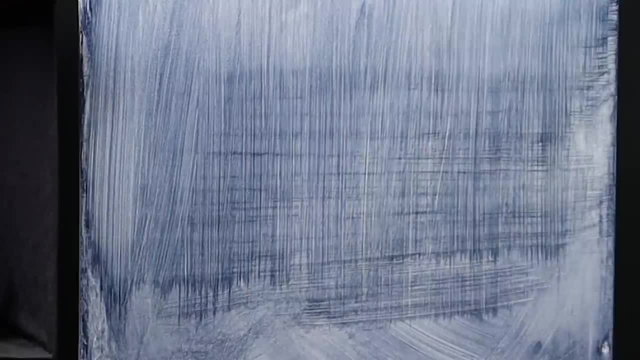 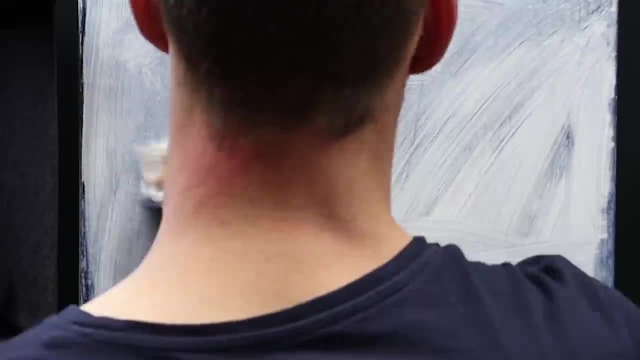 your canvas as your primer and also if you have never used oil before. Acrylic can only be used before oil painting is put on the canvas and not after. Now the fourth option is to do what's called an oil transfer. It's a good way to take. 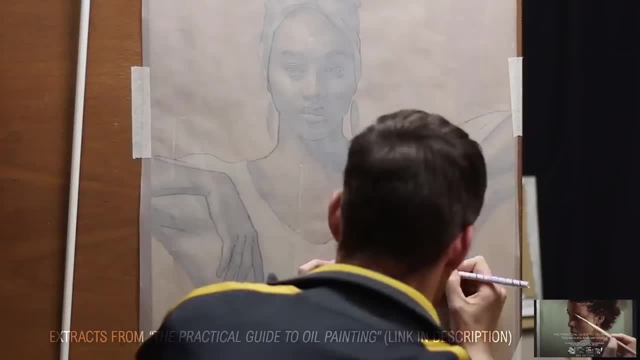 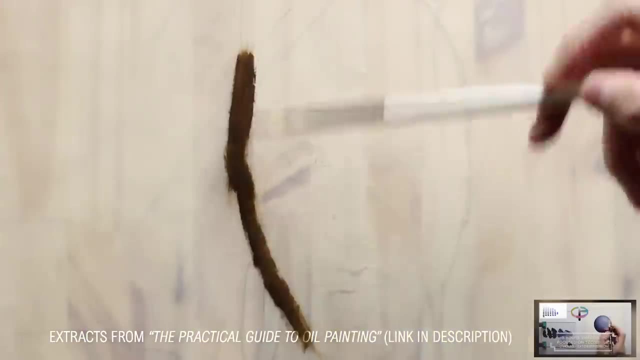 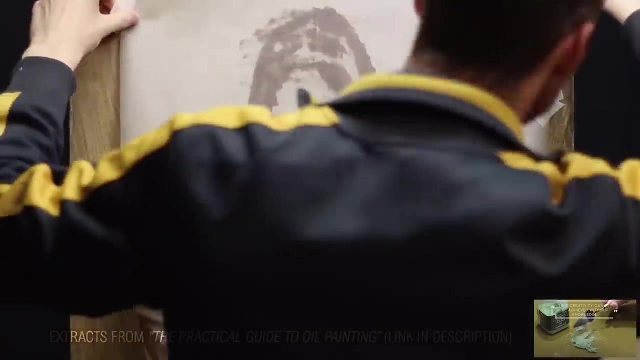 a drawing that you've made separately and start with its outline. First, trace over your drawing with transfer paper. Next turn the sheet upside down and cover the lines with raw umber paint just straight out of the tube. Apply it on the canvas without pressing with your hands and then simply trace over the 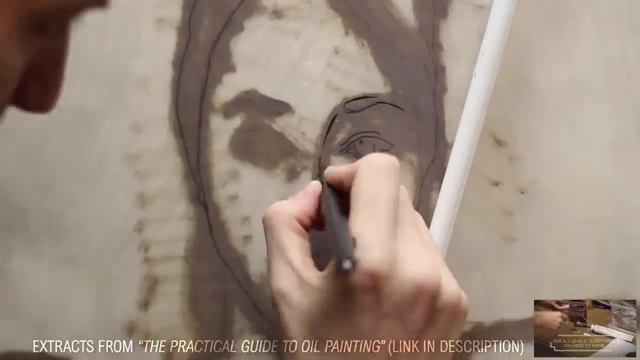 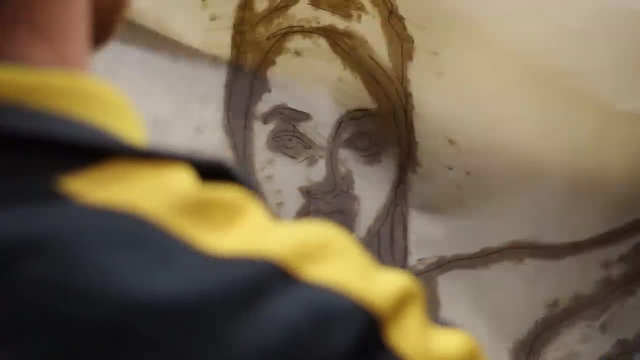 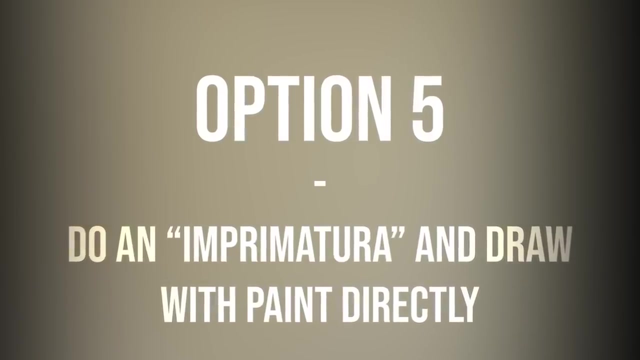 outline again without touching the surface with your hand. You can let it dry, because raw umber dries pretty quickly and you can tone it afterwards, or you can also tone the canvas before. And option five is to draw an imprimatura with paint directly. 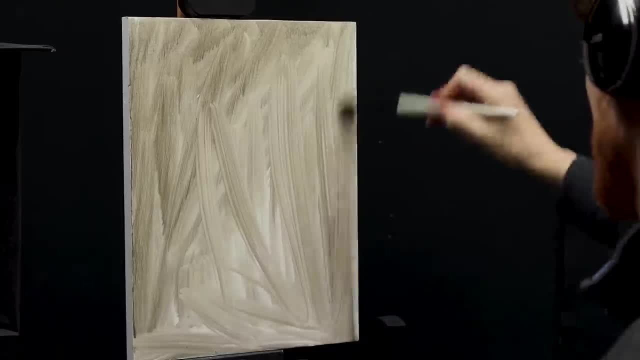 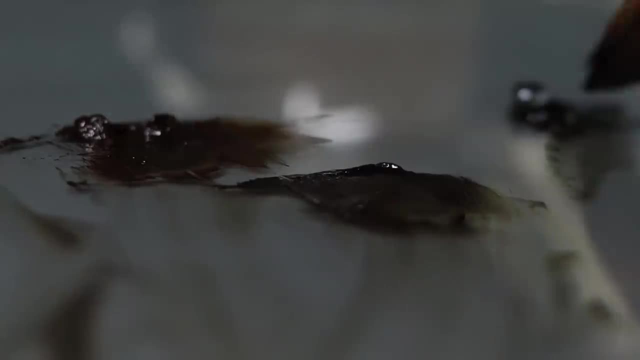 Let's say that it's the more advanced technique, because the drawing, the toning and the construction are all done at the same time. For that you use a wash of solvent like odorless mineral spirits, plus a fast-drying. 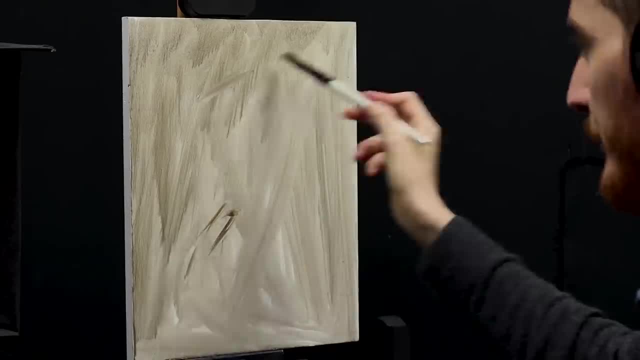 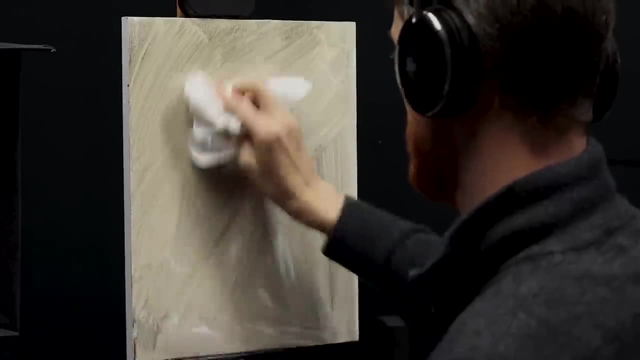 pigment And after that you just start blocking in your drawing with a brush. To erase you can use a piece of paper towel. So the paint is going to be very fluid at first and it gives you time to get the basic position and proportions. 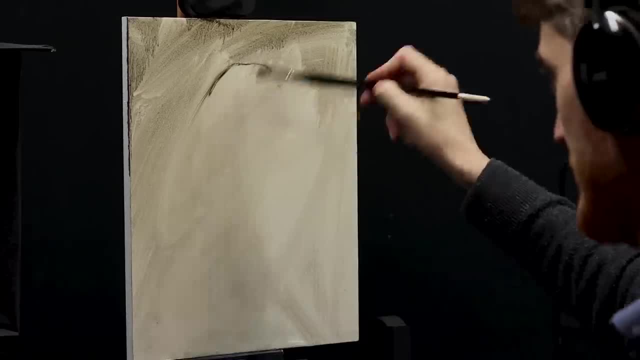 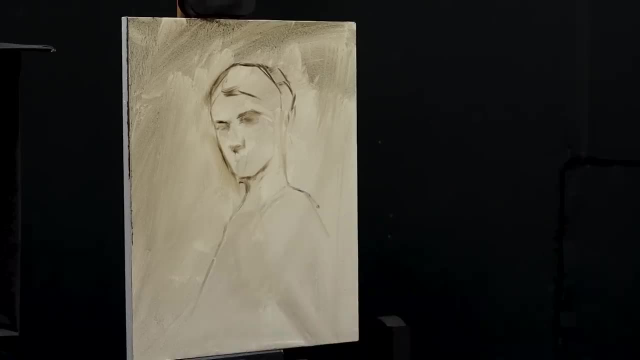 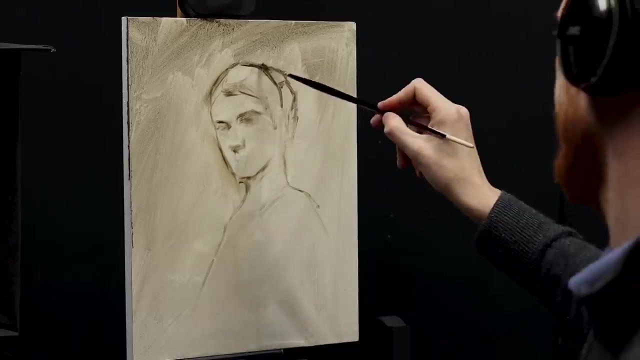 It will slowly dry in a couple of hours and just when your drawing starts to need more precision and accuracy, you can use less solvent And take more of the pure pigment to trace darker lines. So slowly as the paint dries, you reach more accuracy in your painting and things evolve. 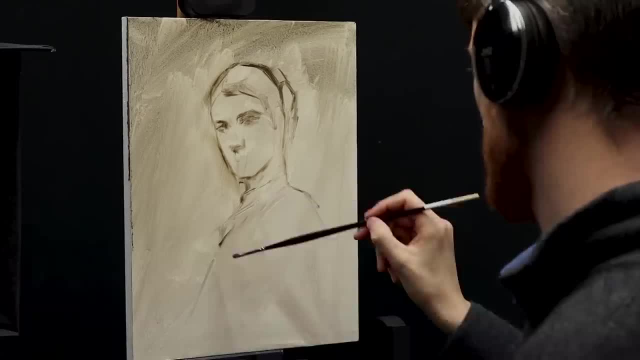 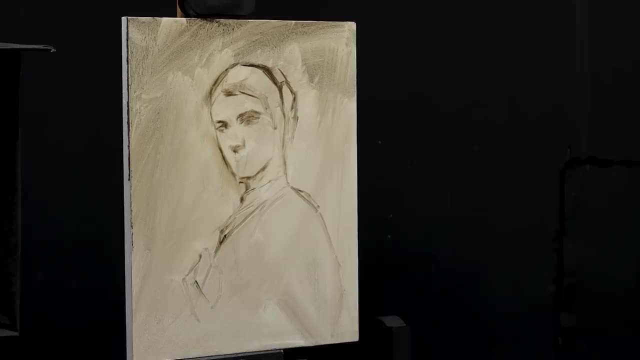 this way. The good thing about this method is that the construction of your painting will follow a very spontaneous and organic process where you slowly build the painting with paint and little by little, it evolves to create a better, more natural look, And that's what I'm going to show you in this video. 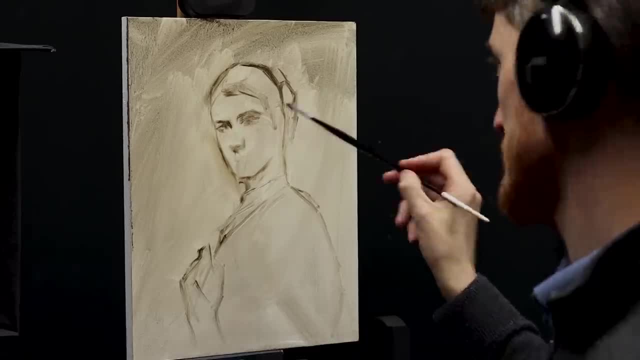 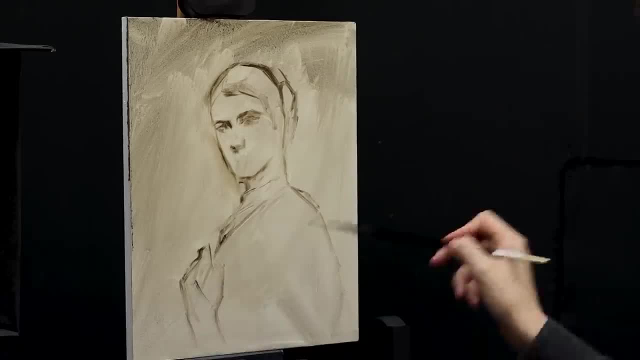 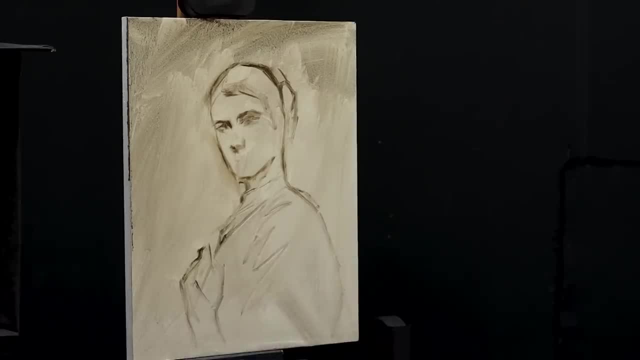 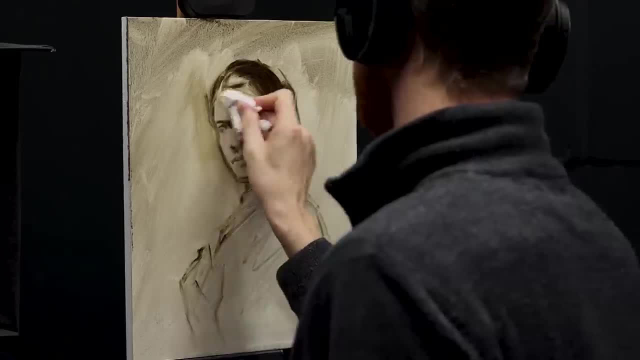 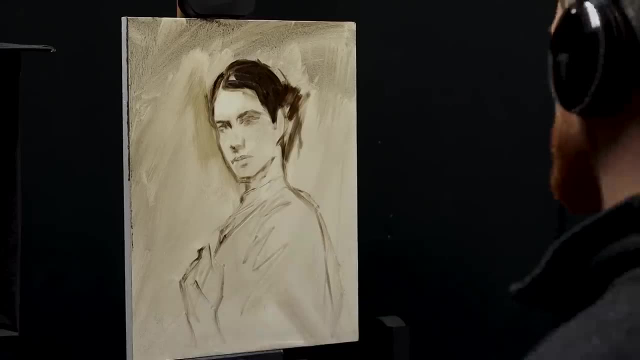 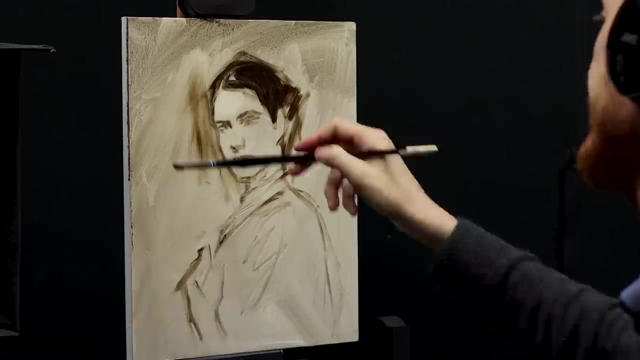 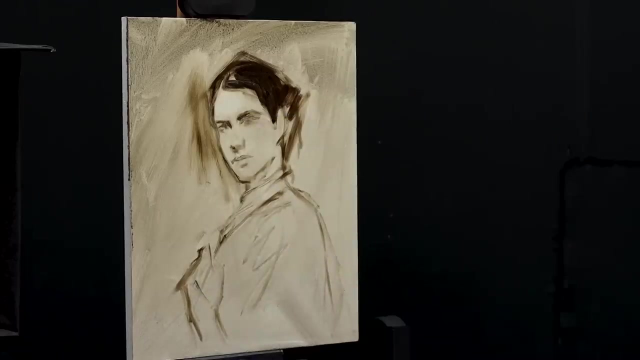 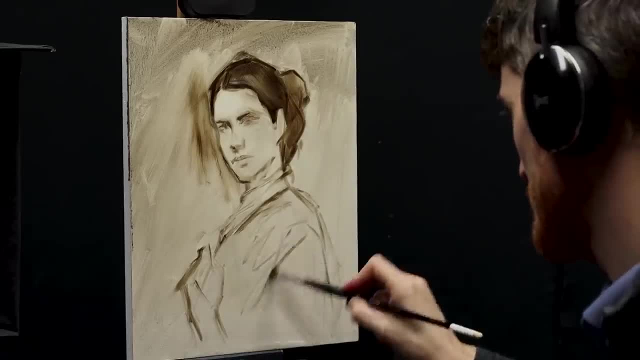 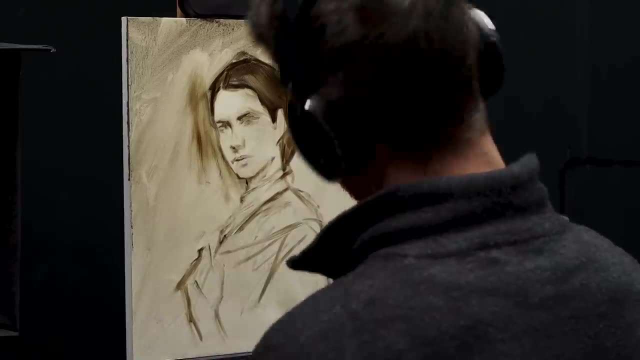 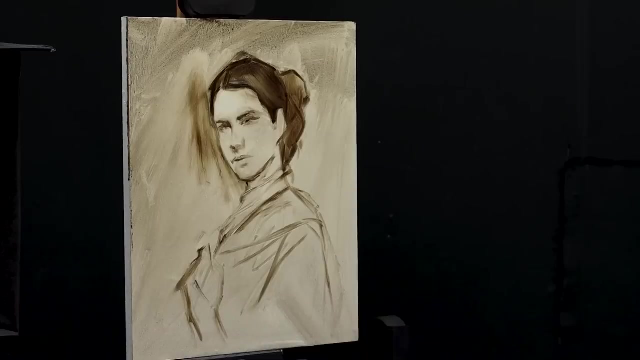 it's not very easy to erase because, first of all, you feel really connected to your painting from the very first moments. plus, you do everything at once: the outline, the drawing and the composition. If you're not really confident in your drawing skills, this might not be the technique for you, though. 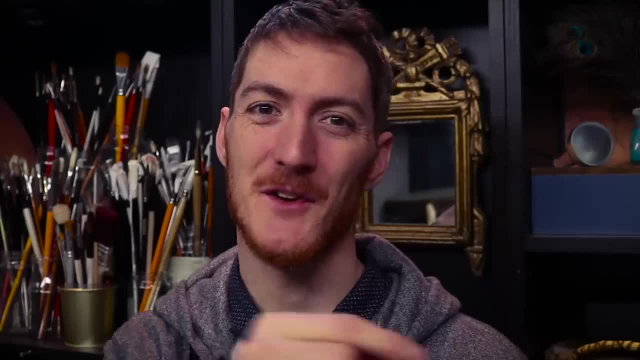 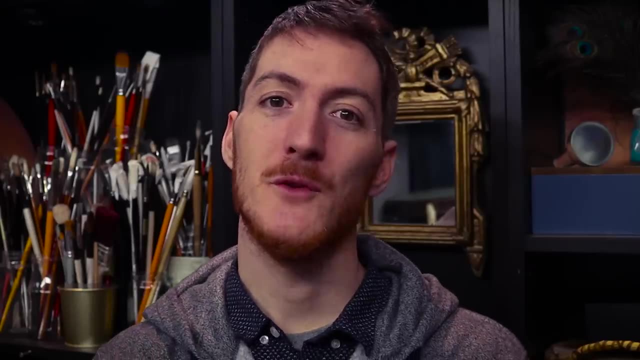 Alright, that's it for this video. How do you generally start with your paintings? Leave a comment down below. You can also reach me on Instagram. if you don't already follow me there, you should. A big thank you to all my patrons on Patreon, your.